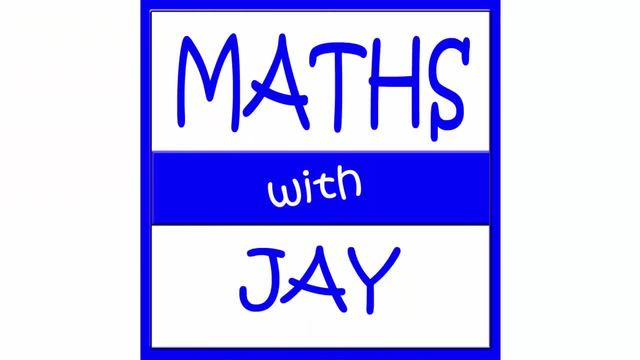 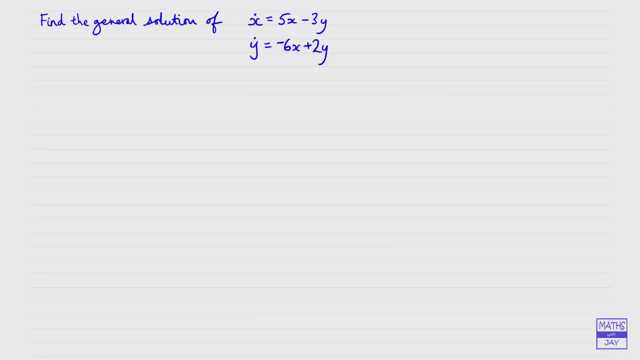 Hello and welcome to Maths with Jay. So we're going to solve this system of equations, differential equations. Before we do that, let's just make sure that we know what we've got here. When we write x dot, that means we're differentiating x with respect to t. 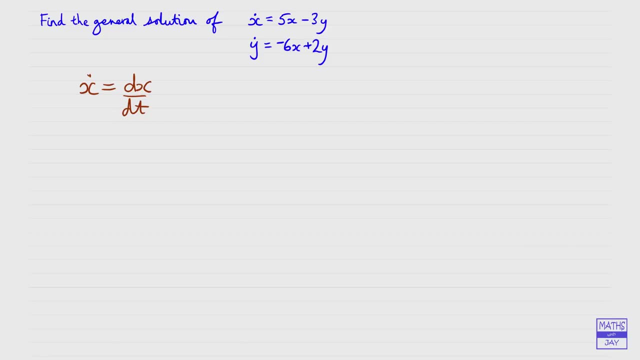 So x dot is dx by dt and similarly y dot is dy by dt. And when we're asked to find the general solution of these equations, that means that we're trying to find both x and y as functions of t, And what we're going to do now is write this in matrix: 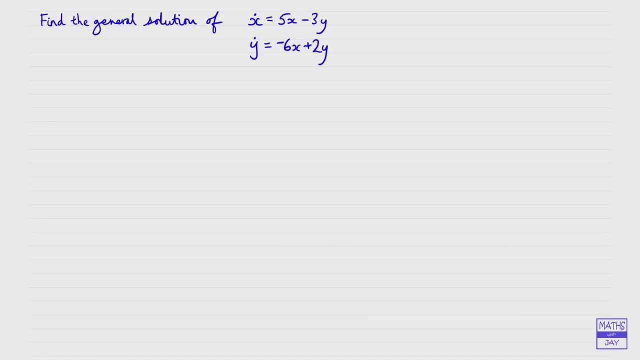 notation. So let's write the derivatives as the column vector. So we've got x, dot, y, dot and now the coefficients multiplying the x's and y's, that will be a two by two matrix. So we've got five negative, three negative, six and two, and that's multiplying the vector x- y. 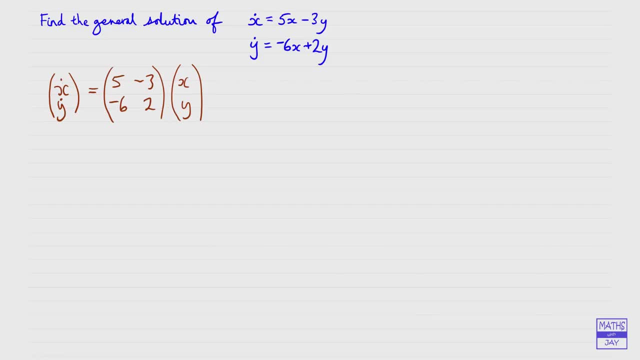 So that's the equivalent to what we've got to solve, and, in fact, the way to solve this is to look at a two by two matrix and to write down its eigenvectors and eigenvalues, And we've already done this, in fact, in an earlier video. 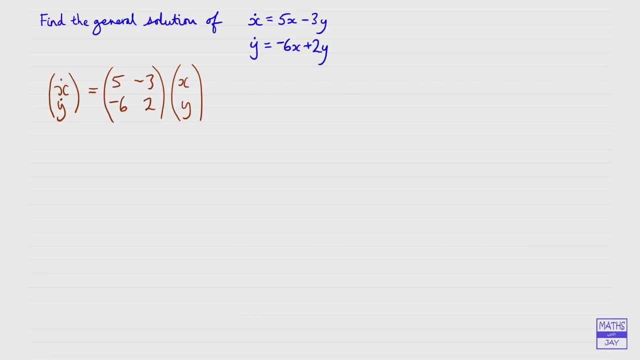 So let's write down what the eigenvectors and eigenvalues are. So we found that our eigenvalues, lambda one and lambda two, were negative one and eight And the eigenvector corresponding to the first eigenvalue, I'll call that x one. 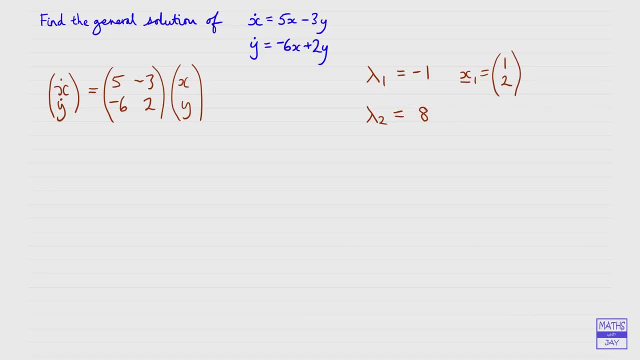 was one two, and the eigenvector corresponding to the second eigenvalue is one minus one. So those are the eigenvalues and eigenvectors for this matrix And we can write down the general solution in vector notation of these equations or of this matrix. 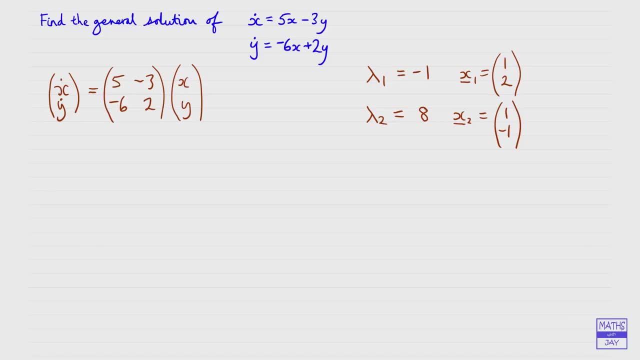 equation. So let's write down the general solution in vector notation of these equations or of this matrix equation, And that is, let's just write it over here- Our solution in vector notation. So x and y is equal to an arbitrary constant c. 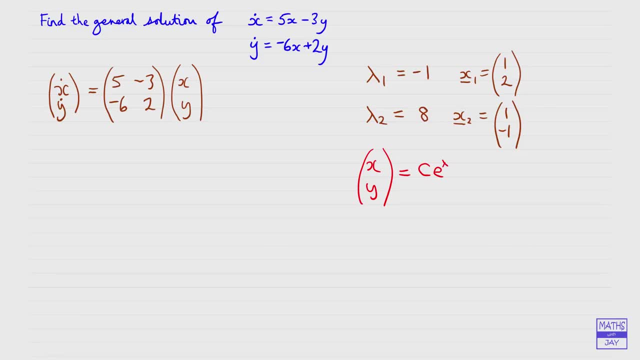 multiplied by e to the power of lambda one multiplied by t, And then that multiplies the first eigenvector, so x one, x1. and similarly we've got another arbitrary constant, d, this time multiplying e to the second eigenvalue, so lambda 2 multiplying t, and that multiplies the eigenvector associated. 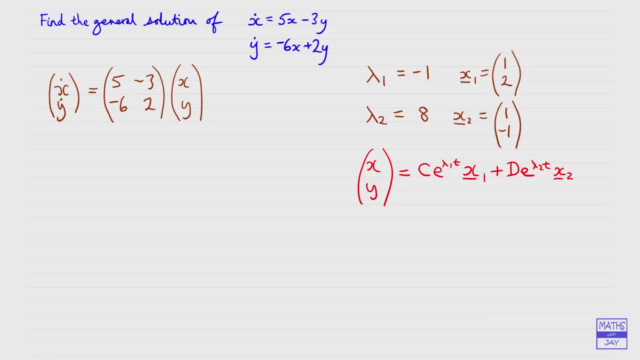 with that eigenvalue. So that's our general solution. so now all we need to do is to substitute in lambda 1, lambda 2, x1 and x2 and we'll have our answers. So we've got that. our solution is: xy is equal to the arbitrary constant c times e, to the power of negative 1 times t. so that's. 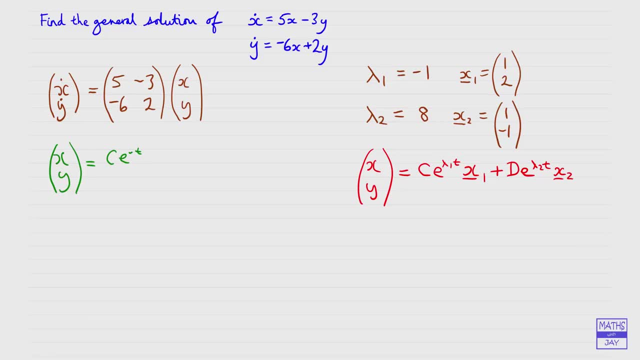 minus t, and then that's going to multiply the eigenvector associated with the eigenvalue minus 1, so that's 1: 2.. And then we've got our next arbitrary constant, d multiplying e to the power of our second eigenvalue, so that's lambda 2 in this. 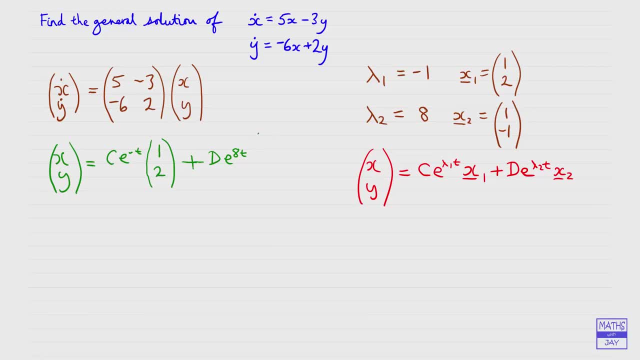 case it's 8. so e to the 8 t and the eigenvector associated with 8 is 1 minus 1.. So that's the solution in vector notation. So let's now write the solution in ordinary notation. so x, looking at the top line, is going to be c times e to the power of negative t. 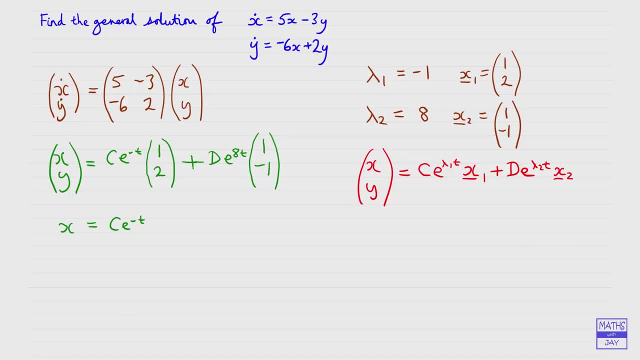 times 1, so that's c e to the negative t, and then d times e to the 8 t multiplies 1, so that's d times e to the 8 t. and then, looking at the second line, y is c times e to the minus t times 2, so let's bring the 2 out. 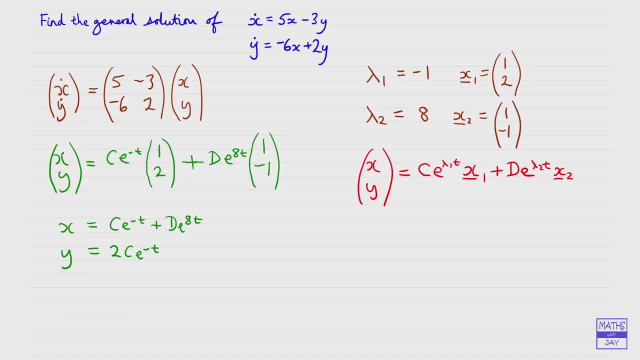 in front, and then we've got d times e to the 8t times negative 1, so let's bring the negative in front. so we've got d times e to the 8t there, And then it's a good idea to check your answers. 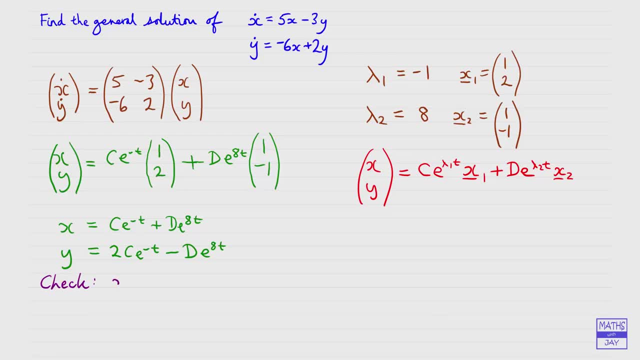 So checking. let's check the x answer. So if we differentiate our answer with respect to time, work out dx by dt, we get minus 1 times c times e to the minus t. so that's minus c e to the minus t. 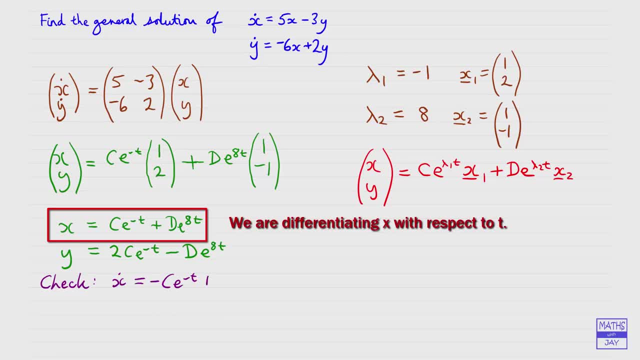 And then, differentiating the e to the 8t, we'll get 8, so that's going to be plus 8 times d e to the 8t. And then we know that that should be equal to 5x minus 3y. so let's write down what that's equal to. 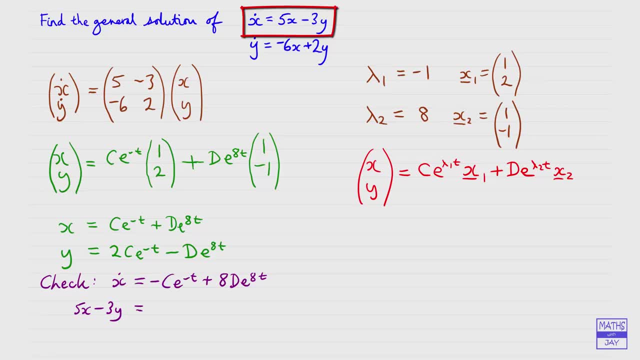 So. So 5x minus 3y is equal to 5 times c? e to the minus t, plus d e to the 8t. We're subtracting 3y and y is equal to 2c e to the minus t, minus d e to the 8t. 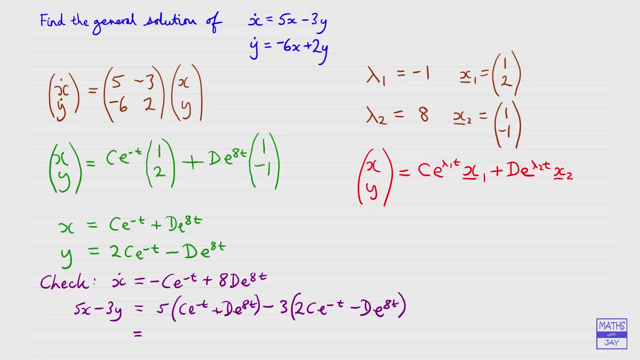 So that's equal to. Well, we could take c outside a bracket and then we have got 5 from the first bracket and then minus 3 times 2, so that's going to be minus 6, and then that will be e to the minus t. 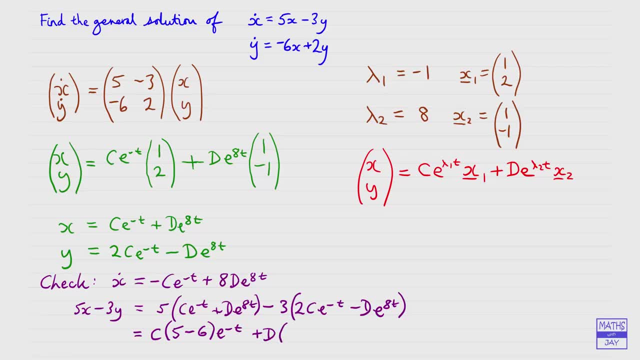 And then plus d from the first bracket, we've got 5, and then minus 3 times minus 1, so that's plus 3.. And that's e to the 8t. So that's going to be equal to minus c, e to the minus t, plus 8d, e to the 8t. 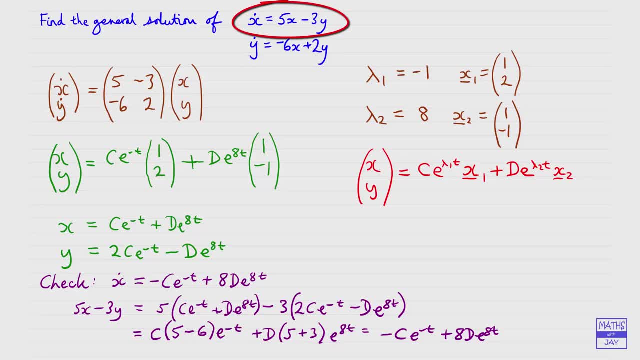 And so that is equal to x dot. so it looks like we're right. And of course you can check y dot in the same way. We'll check y. Yeah, work out what dy by dt is and check that you do get minus 6x plus 2y. Thank you.